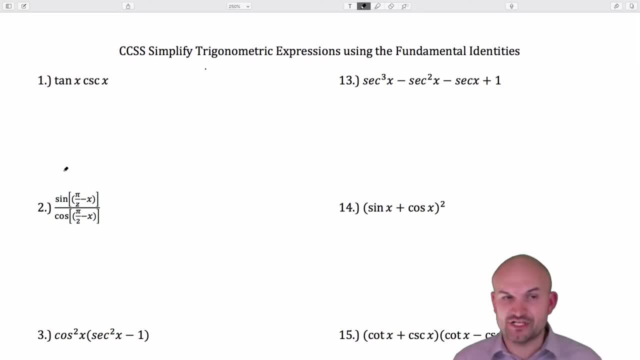 typically we either want to apply the operation that is given or we're going to want to try to reduce it to one trigonometric function or number. So one thing that's kind of helpful is when you don't see, like you can't multiply this. you know it's not like x times x is x squared. 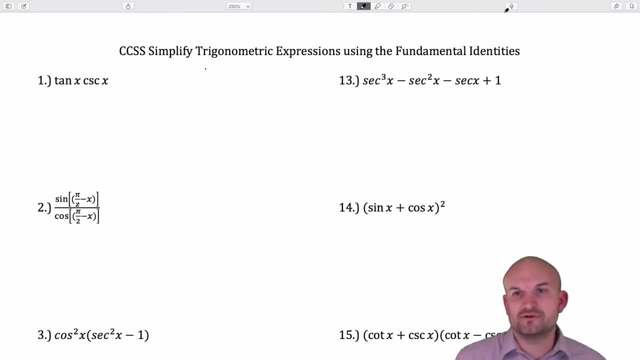 So one thing that's usually kind of helpful- let me get to my red- is to go ahead and write things in terms of sines and cosines. So I'm going to write tangent in terms of sines and cosines using the quotient identity. 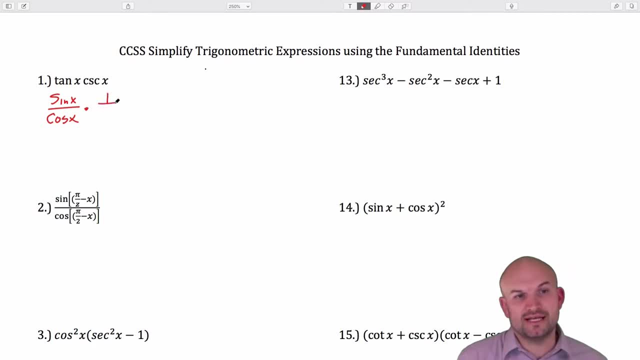 And I write cosecant in terms of the reciprocal identity. You can see that now the sine divided by sine via the division property is going to divide to one. Therefore, that's just going to leave me with one over cosine of x, which I can simplify to just secant of x. So you: 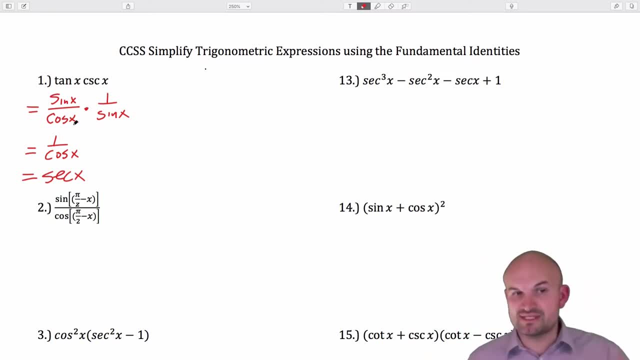 can see that by multiplying them. basically, what we want to do typically when we're simplifying is we're going to be looking for items to divide out. Now, that doesn't happen for every one of these problems, but you can see that's kind of like our general idea to simplifying the expression. 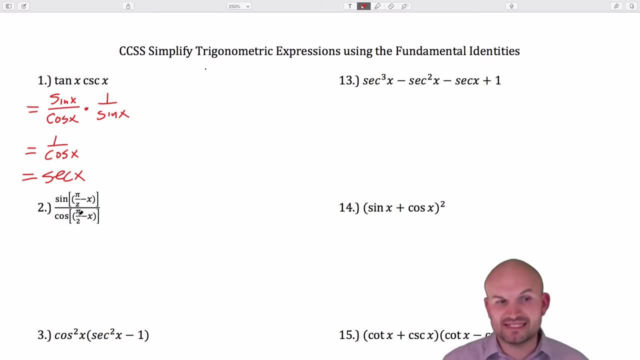 The next one is: we have the sine of pi halves minus x, as well as cosine of pi halves minus x, And what this represents is the co-function identities. So what I'm going to do here is I'm just going to apply the co-function identity immediately. So remember, these are basically. 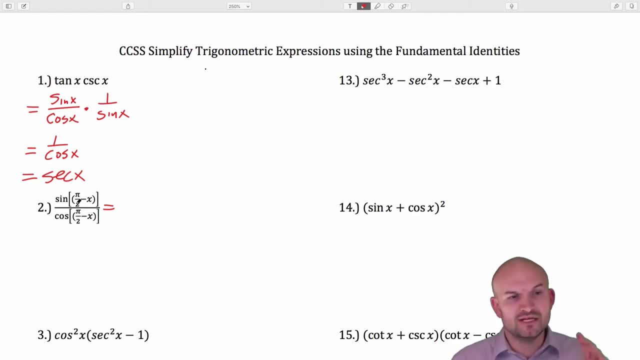 the way that I have these memorized is like transformations of a function. So if I was going to take the sine graph and I was going to transform it right, the only other graph it could look like would be the cosine graph. And if I was going to take the cosine graph, 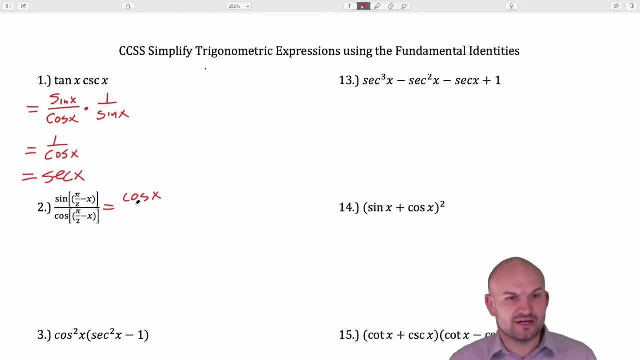 and I was going to apply transformations to it. the only graph that could look like would be the sine graph, So in this case I'd have cosine of x over sine of x which, using my quotient identities, I can see can be represented as a cotangent of x. 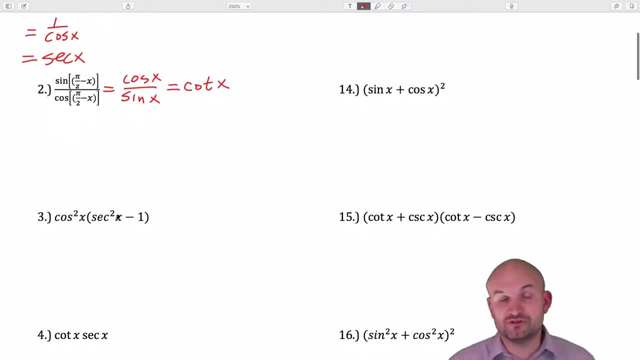 Now the next one might be: you might want to look into distributing, which you definitely could do. However, it's also important for us to recognize our Pythagorean identity here, And if you recognize, actually you know well, we could do it both ways. Let's do the first way of just multiplying. 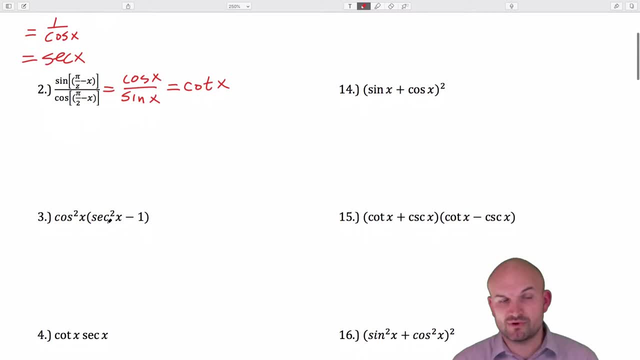 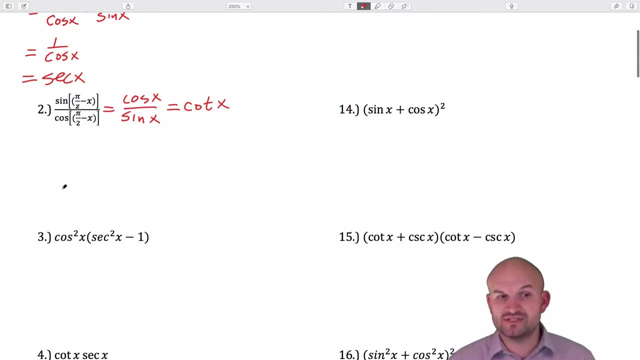 this through. So if I was going to multiply cosine squared of x times secant squared of x, recognize that cosine and secant are reciprocals of each other, right? As we already mentioned, secant can be rewritten as one over cosine. So if secant squared can be written as one over, 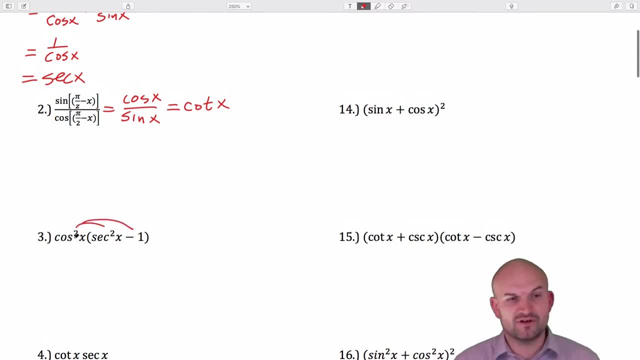 cosine squared. So if I was to distribute this, I would have cosine squared of x times secant squared. So if I was to distribute this, I would have cosine squared of x times secant squared of x. So if I was to distribute this, I would have sine squared of x is one minus a cosine squared of x. 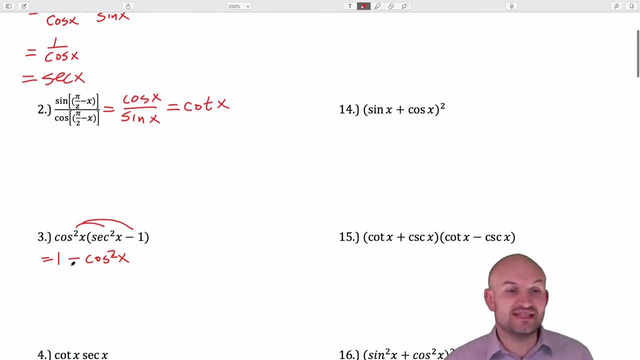 Now what you can see here is one minus cosine squared of x, using the Pythagorean identity. using the Pythagorean identity is going to equal to sine squared right, Because, remember, sine squared plus cosine squared equals one. So if you just subtract cosine to the other side, 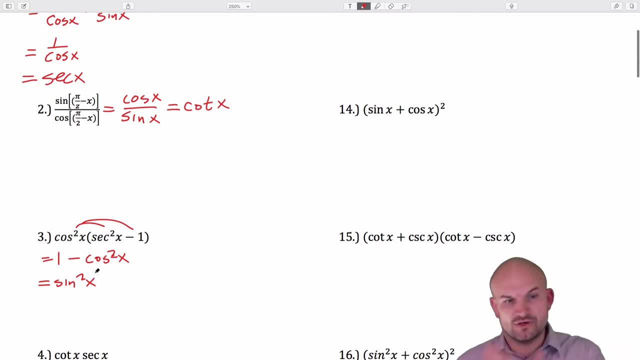 you'd have: sine squared of x equals one minus cosine squared of x, So you can see how it's equal to sine squared. The other way you could have done this is you also could have just rewritten this using the Pythagorean identity as tangent squared of x. 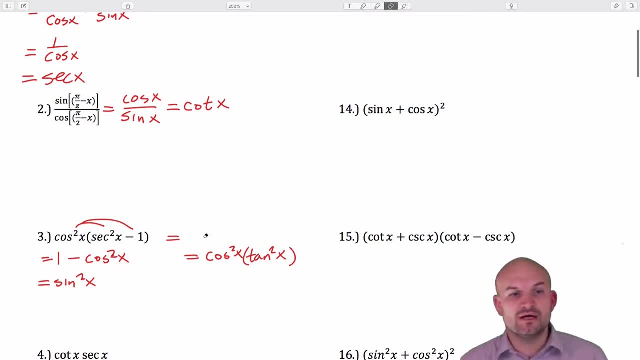 So you could have recognized that secant squared of x is equal to, or secant squared of x minus one is equal to tangent squared of x, And therefore cosine squared of x times tangent squared, because, remember, tangent is sine over cosine, So therefore cosine denominator. 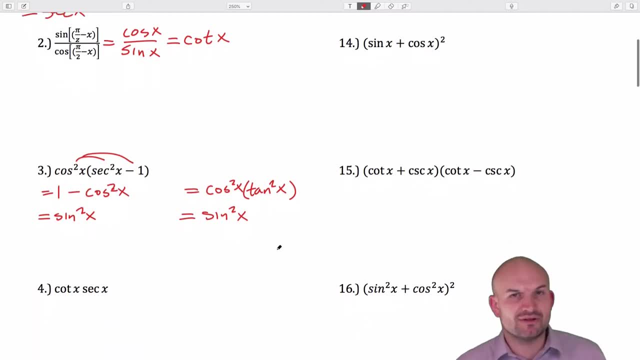 cosine the numerator, you'd just be left with a sine squared of x. So a lot of these problems. there's always going to be multiple ways. I'm not always going to show you every single way that you could do it, But in this case I came up with an opportunity. 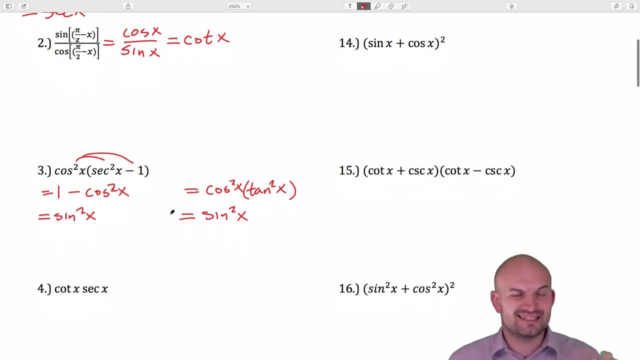 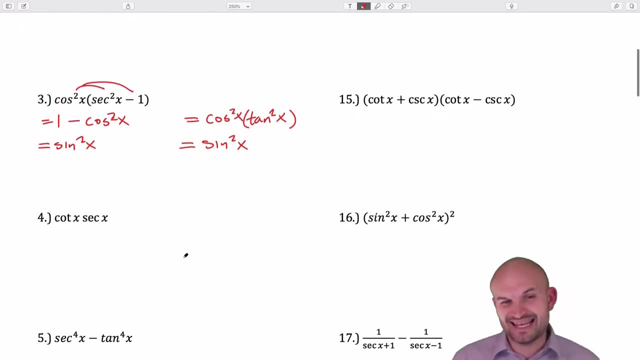 that I said. well, actually multiplying or using Pythagorean identities is kind of like equal, So I want to show you both ways. In the next example we have cotangent of x times secant. Again, I'm not recognizing anything that divides out there, So therefore I'm going to write them. 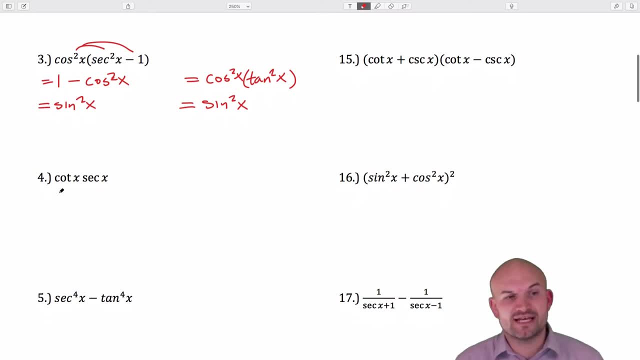 in terms of sines and cosines and see what can happen here. So I can write cotangent as cosine of x over sine of x and secant as one over cosine of x. See, the cosines are going to divide out. That's going to leave me with a one over a sine of x. 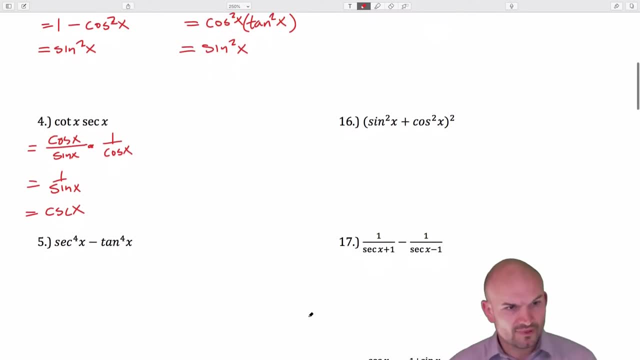 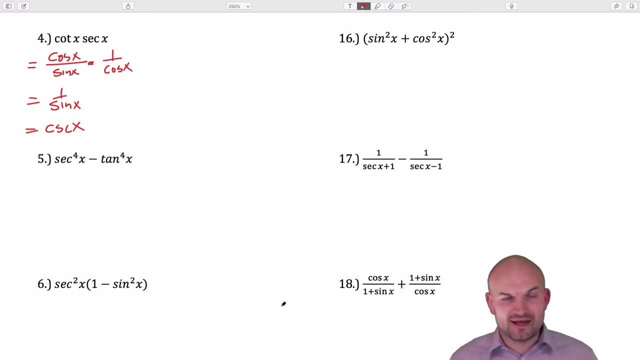 which is equal to a cosecant of x. The next problem is a secant to the fourth of x, minus tangent to the fourth of x. Now, the one thing I recognize, though, is this is a binomial raised to the fourth power, And immediately I think of the difference of two squares. Now again, 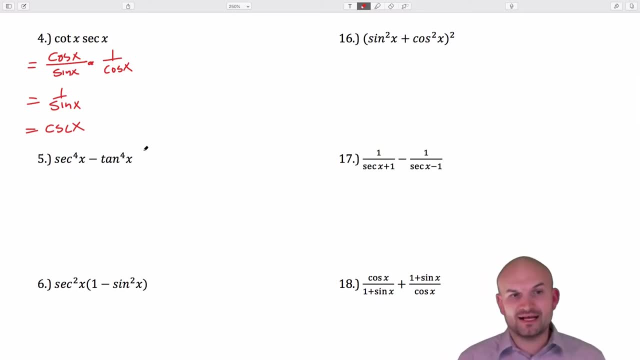 four is not a square right, It's not squared. However, I recognize that relationship. I have something to an even power minus something to that same even power. So, therefore, if you were to think about this like we did this in polynomials, actually, if I had a to the fourth, 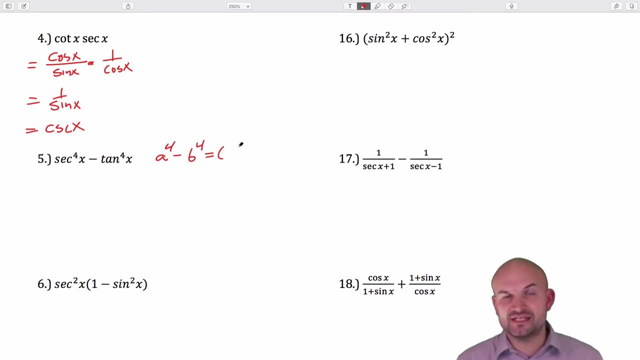 minus b to the fourth. I can factor that using the same factoring process of difference of two squares as a squared minus b squared, times a squared plus b squared. So when you recognize like a factoring relationship, that's the exact same thing we're going to want to do here with. 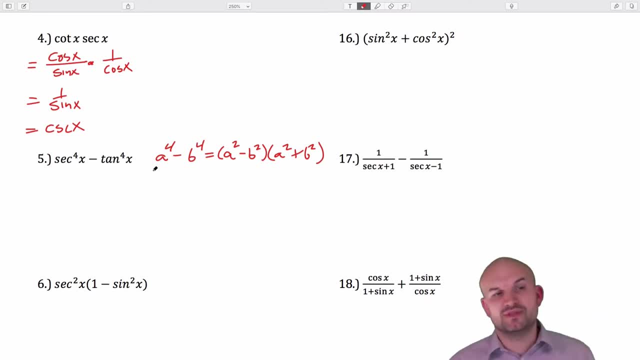 this problem. We're going to want to apply factoring to this expression, So therefore, I'm going to write this as secant squared of x minus tangent squared of x times secant squared of x plus tangent squared of x. Now you might be wondering why would we want to do that? That kind of looks, kind of. 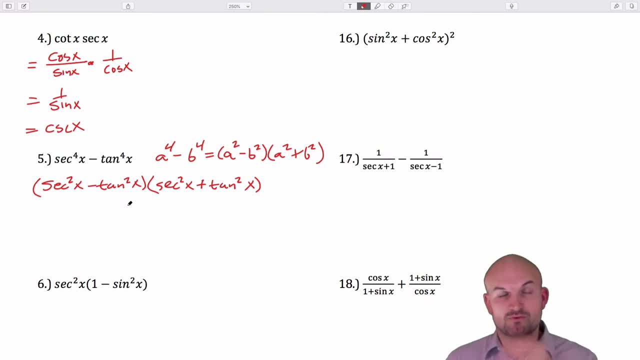 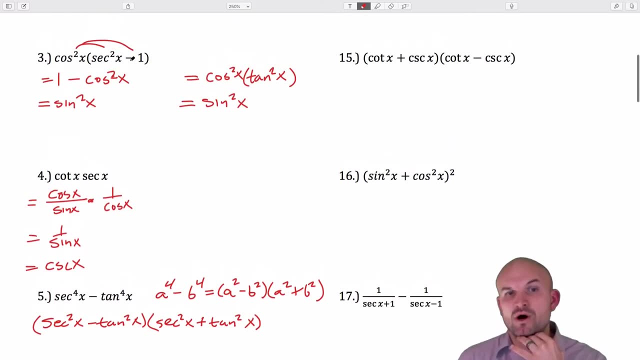 simplified. Well, you know, one of the things that's nice about this is when we have things in terms of squared, we can write them as a single trigonometric function. So remember, we said that a secant squared of x minus 1 is equal to tangent squared. So what I'm going to do is: 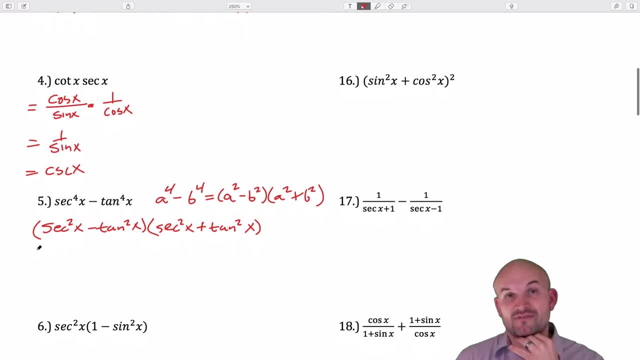 whenever I see tangent squared, I'm just going to write that as a secant squared of x minus 1.. So, therefore, I have secant squared of x minus a secant squared of x minus 1, and then times a secant squared of x plus a secant squared of x minus 1.. 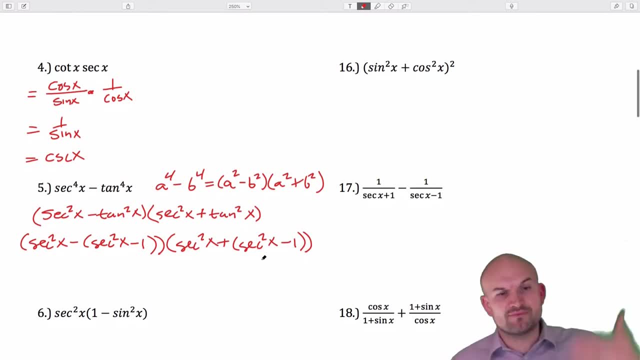 Okay, so now what I've done is I've just rewritten the expression all in terms of of secants or, I'm sorry, in terms of tangent, And actually, yeah, I don't know why you'd want to do it in secant. You could do it in secant or in terms of signs, if you want to. Well, as I. 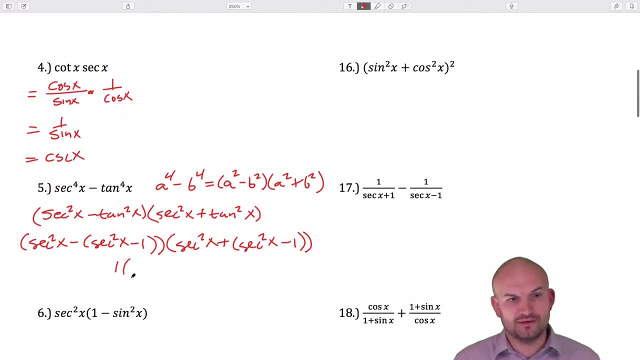 distribute. here I basically just get a positive 1, because secant squared minus secant squared of x is just going to be a positive 1.. And then here I'm going to have a 2 secant squared of x minus 1.. 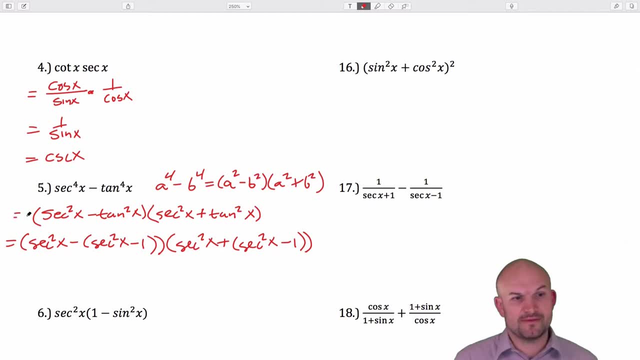 So therefore, this answer: actually, when you just go ahead and simplify, this becomes a 2 secant squared of x minus 1.. And then again, if you wanted to write it in terms of tangent, you could just replace secant. 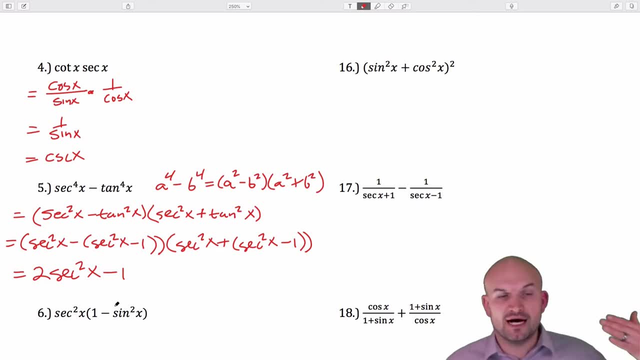 squared of x, with, you know, tangent squared plus 1.. And then you could go ahead and simplify it and you'd get the other expression as well. So you know, I just picked one. I just picked to decide to rewrite tangent in terms of secant, because that's something we have already. 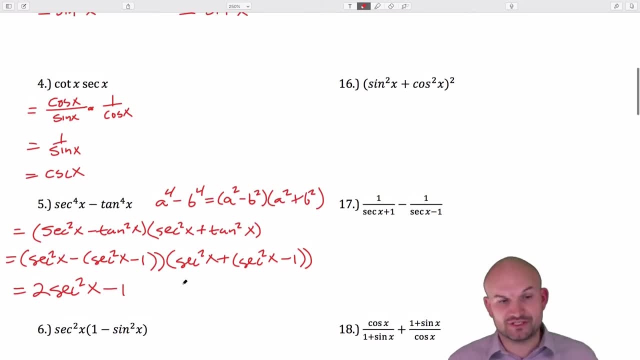 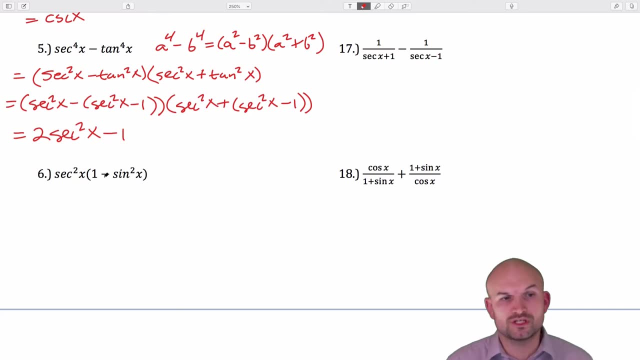 we'd already shown. However, you could also write everything in terms of tangent. For the next example, again, we have this other opportunity to either multiply or just simplify. I recognize like that Pythagorean identity. you know, the 1 plus your sine squared plus cosine squared equals 1.. 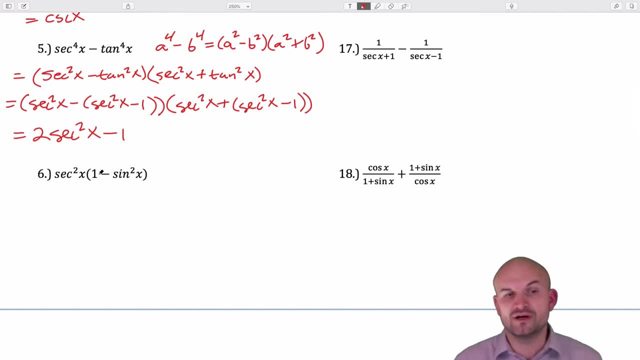 I think it's just really important to make sure you understand. So therefore you can see that if you subtract sine squared to the other side, that's going to equal cosine squared. So in this case I have secant of x times cosine squared of x, And then now you can see that I have secant squared of x times. 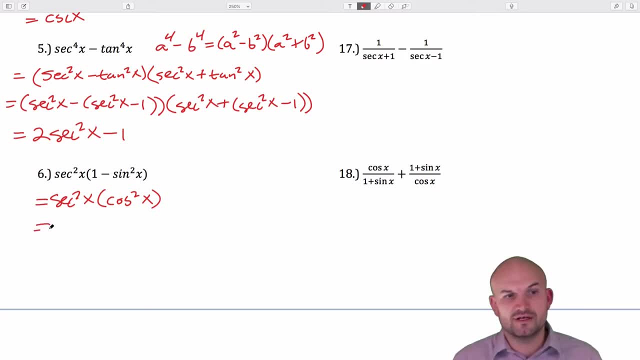 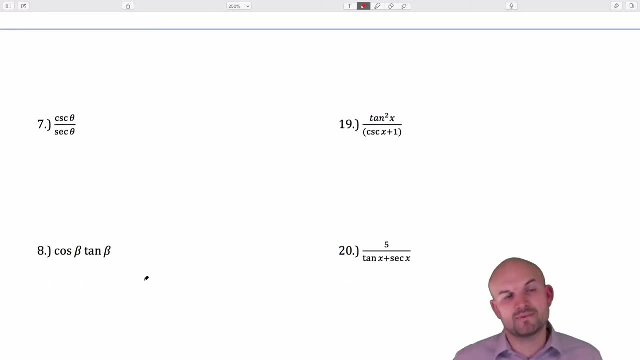 cosine squared of x. Those are reciprocal functions of each other, So that's just going to equal 1.. All right, Moving on down now, let's go and get into a fraction here, or a division. So we have cosecant of theta divided by secant of theta. Now again, the best thing, I think, that I like to remember. 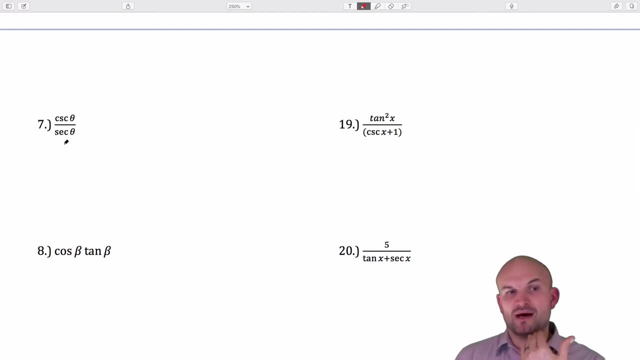 here is: rather than dividing, I prefer to multiply by the reciprocal. So in this case, rather than writing this as cosecant of theta, divided by secant, I'm going to write multiply this times and multiply the reciprocal, Because again like to think about it this way and actually let me go through this a little. 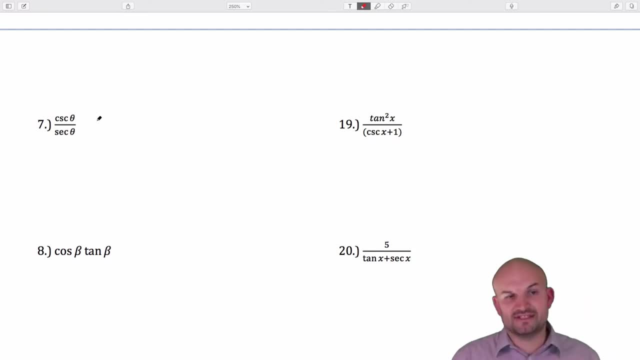 bit quicker or a different way. If I wanted to get secant off the denominator, I would multiply by its reciprocal, which is 1 over secant of theta. Now, using the reciprocal identities, I recognize that's the same thing as multiplying by cosine, right? But again, what I really have here is: 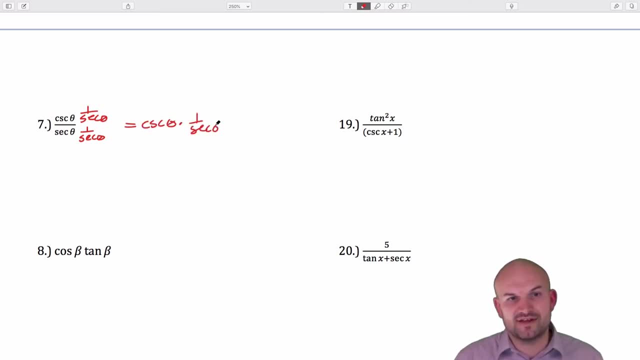 cosecant of theta times 1 over secant of theta. Now again, instead of writing that, you could just think about this and say, all right, instead of writing this as a division problem, I'm going to write this as a. 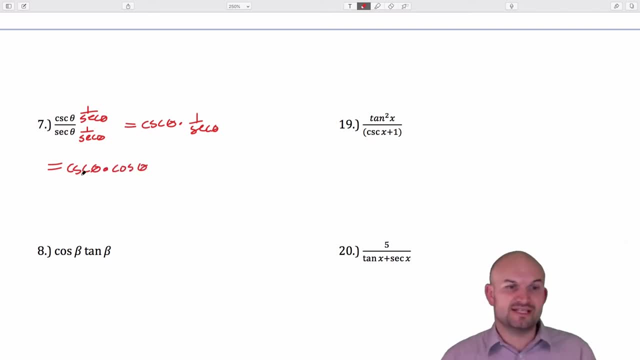 multiplication problem. Now again, you might not recognize this cosecant of theta times cosine of theta. So therefore you might need to probably need to rewrite cosecant of theta as one over sine times cosine of theta, And when we do that we get cosine of theta over the sine of theta. 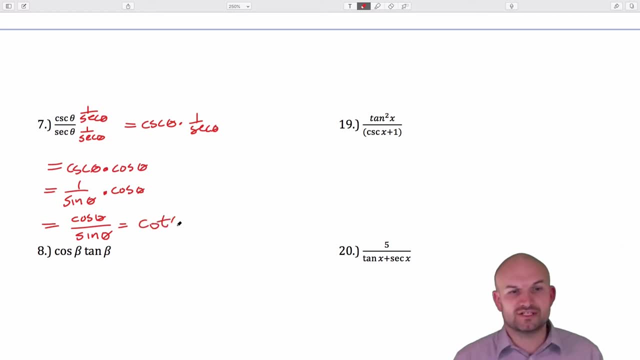 And that is just going to equal the cotangent of theta. Okay, So a lot of times when you have that division, it's going to be best to go ahead and rewrite that as a multiplication problem. Um, all right. Um, so for the next one, we have cosine of beta, times tangent of beta. 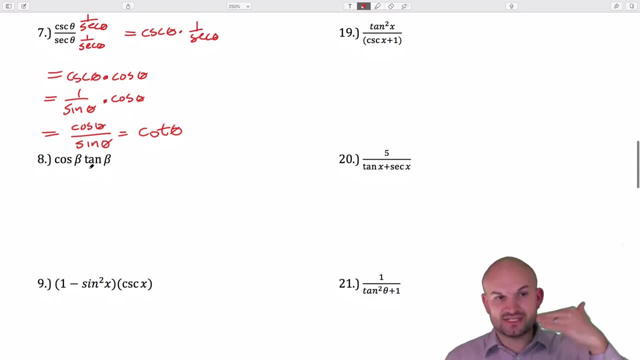 And again, I recognize that tangent can be written as cosine, or sorry, sine over cosine. So, um, that's, um, that's what I'm going to want to obtain to divide out my um cosines. So therefore, I'm just gonna be left with a sine of beta. 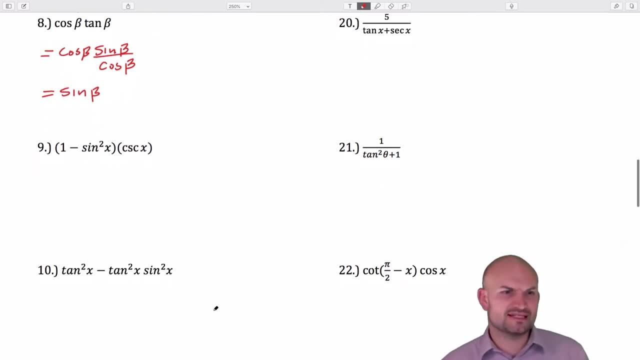 Okay, All right. Next example is I have one minus sine squared. Um, hmm, Interesting why I chose this. So one minus sine squared of X times cosecant of X. Well, that's going to be a cosine squared of X times a one over a sine of X. Now there's a couple. 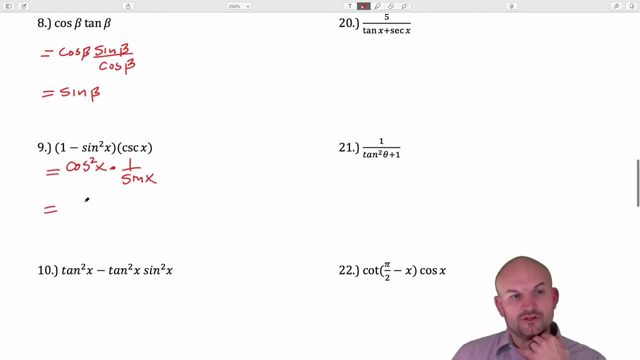 different ways you'll see this being written. Um, you know you could write this as a cosine squared of X, all over a sine of X, right? However, a lot of times in problems you'll see what will happen is they'll separate the cosine of X or cosine squared of X, I'm sorry, to a cosine of. 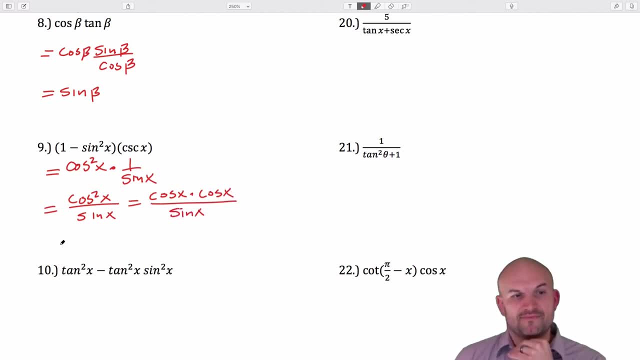 X times cosine of X all over. So that's a cosine squared of X times cosine of X. So that's a cosine squared of X times cosine of X. So that's a cosine squared of X times cosine of X, And therefore we can decide which cosine of X to group with sine of X, And then we could write the answer as cotangent of X times cosine of X. So it's been a while since I worked on this worksheet, So I don't remember if that's exactly what I was thinking of trying to obtain. Um, and it's not really a more simplified version, It's just another way of writing the problem without it being a fraction. 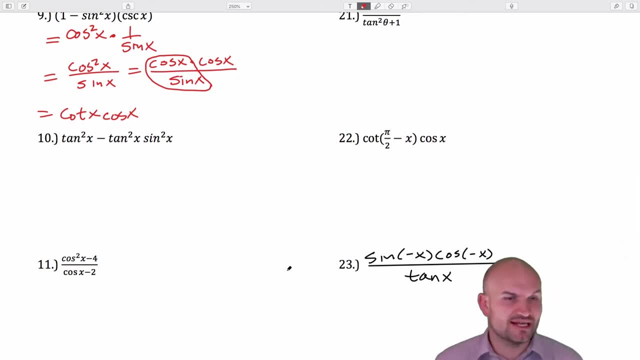 All right. So for question number 10, here this doesn't very look too exciting to go ahead And subtract, So what I'm going to want to do is factor right And you notice that both expressions, whenever you have two expressions that have common elements, think of factoring. 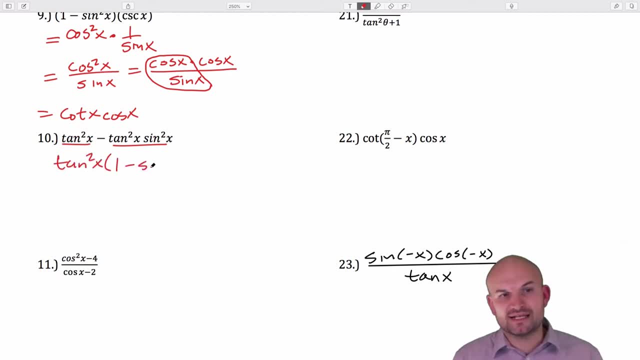 So if I factor out a tangent squared of X, I'm going to be left with a one minus a sine squared of X. Now I recognize one minus sine squared of X is going to be cosine squared, So that's going to be tangent squared of X times a cosine squared of X. 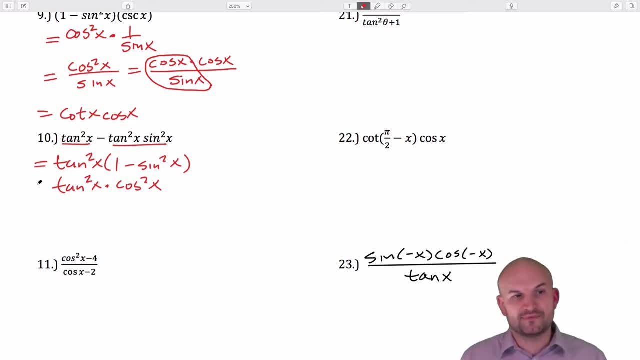 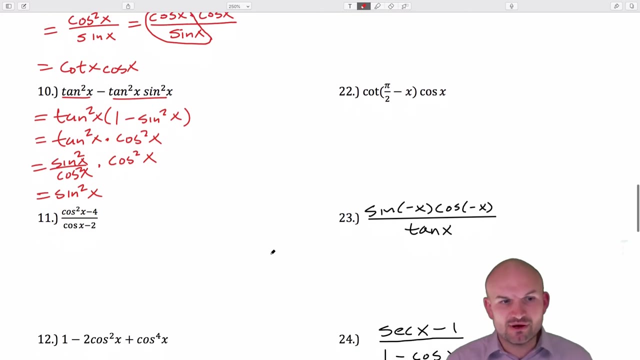 And then again, remember: sine or tangent is going to be sine of X. So I'm going to be left with a tangent squared of X over cosine of X times cosine squared of X. Oh sorry, That's a squared right. So that's going to leave me with a sine squared of X. 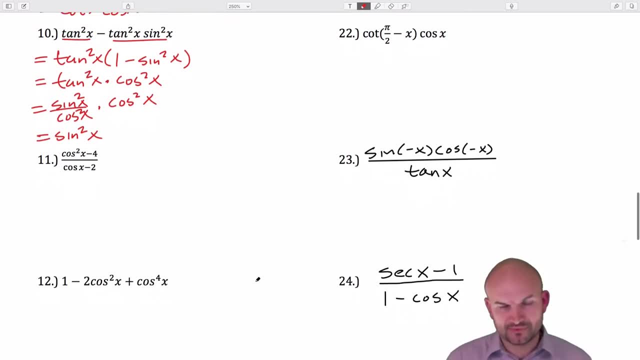 So the next one: we have cosine squared of X minus four divided by cosine of X minus two. Now I see the squared and I want to kind of think again, to use the Pythagorean identities, but um, it's. it's not really going to help me to be able to convert cosine squared into terms of X. 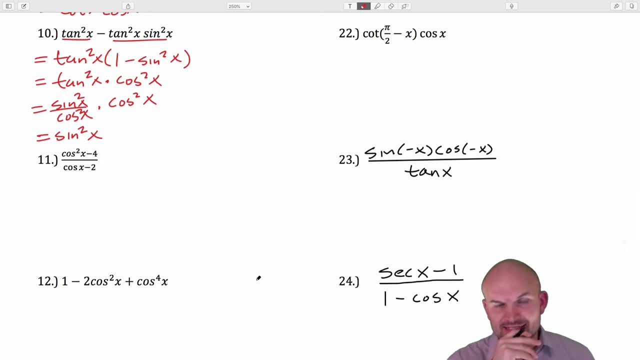 So what I'm going to want to do in this case is: I recognize, though, that these relationships are pretty simple, um, and you can't divide them out, because they're separated by subtraction, But what I do see is I see again another representation of the difference of two squares right. 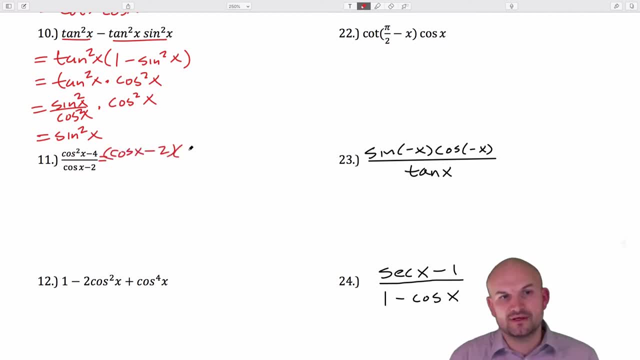 I can rewrite this as cosine of X minus two times cosine of X plus two. Then over here I have the cosine of X minus two. So now I can see that now the quantities are separate by multiplication, Okay, And I can divide those out, which is just going to leave me with a cosine of X plus two. 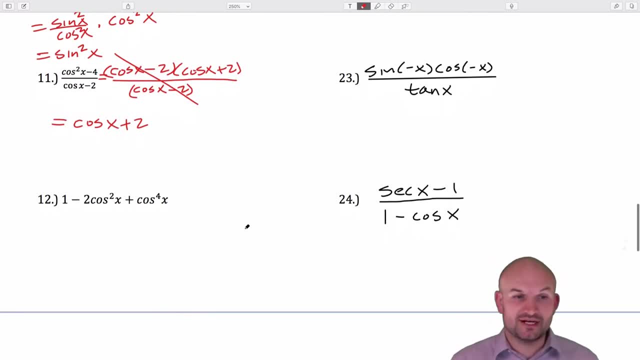 Okay, Um, all right Onto the last one here. Um, I see a trinomial. not everything is cosine, but I see a trinomial. And remember, when I see a trinomial, I'm automatically going to be thinking, factoring. 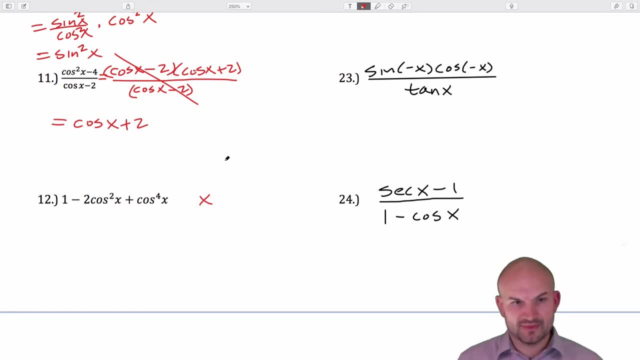 So I'm going to write this in terms of Xs here real quick. So this is just in terms of X to the fourth. So I can factor this X to the fourth minus a two X squared plus one. Now I want to see how is this going to be factorable? 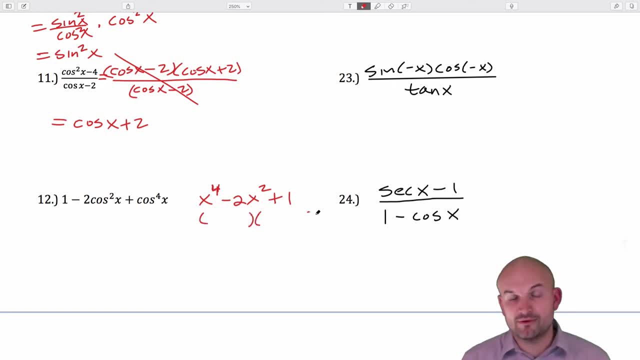 You know what, And remember all quadratics, trinomials, I'm sorry- can be broken down into a product of two binomials. So therefore that'd be an X squared times an X squared. And then what's going to? multiply to give me one, but add to give me negative two. 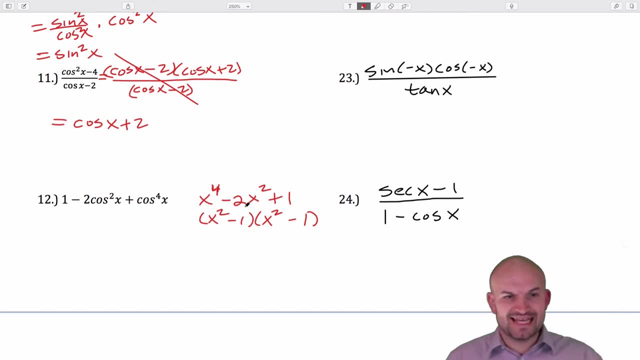 Well, that's negative one and negative one, right? So now I factored with the Xs. Now I'm just going to rewrite that in terms of cosines, So you know, you can rewrite this Typically. I like to rewrite the expression um just in its standard form. 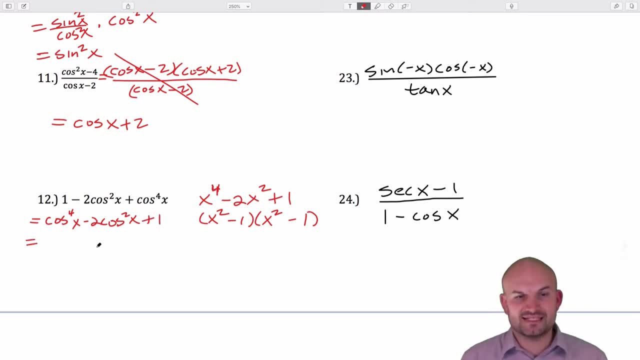 So you can kind of see, but then I can recognize this here to be a cosine squared of X minus one, squared right, Cause you can see that's going to be X squared minus one quantity squared. Um, now it's. it is important to recognize this cosine squared of X minus one. 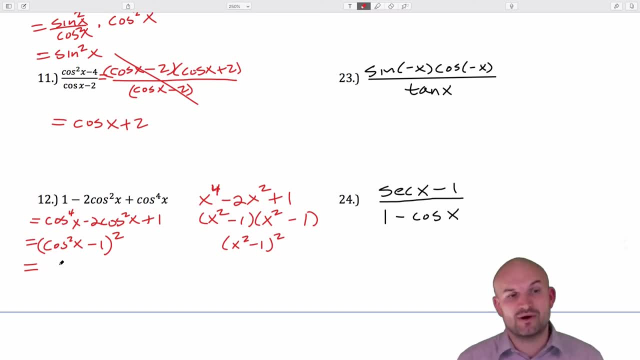 That's going to actually equal negative sine squared, So I can actually write this as a negative sine squared of X squared. Well, if I had negative sine squared, negative sine squared times negative sine squared, that's actually going to equal sign to the fourth of X. 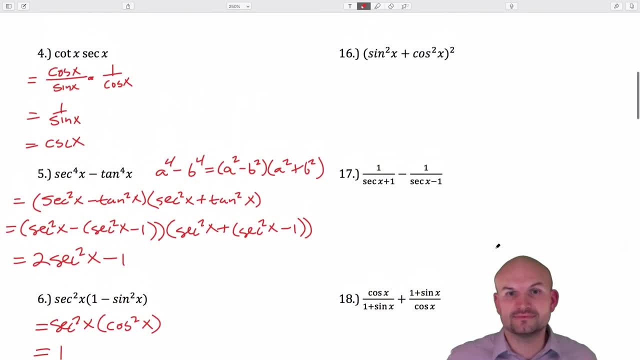 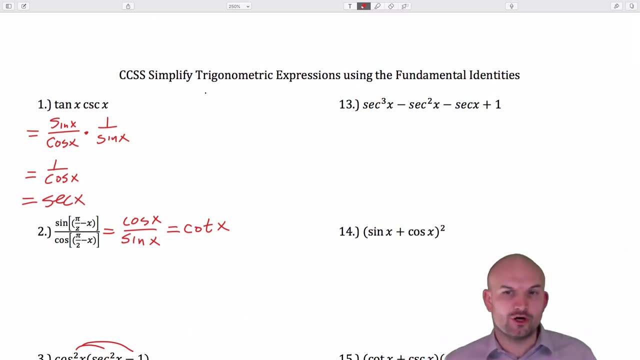 All right, let's go and work on our next round here. Next set of problems. So again we have another problem where we have a lot of secants, right, But in this case we have a polynomial with four terms, or not really polynomial. 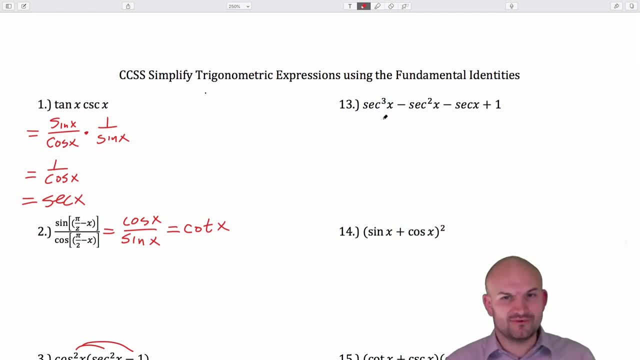 I'm sorry, an expression with four terms, So I can't, you know, I don't really want to look to combine these, I've actually subtracted them. But what I do realize I could do is again factor by grouping. 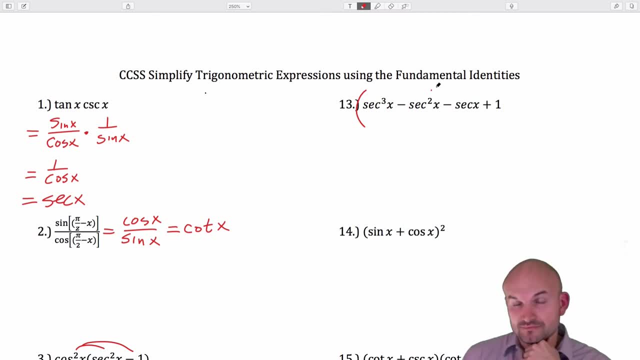 And remember, factor by grouping. What we're going to do is you can just kind of write a plus sign here, So you're not actually multiplying them. But what we're going to do here is group the first two terms and group the second two terms. 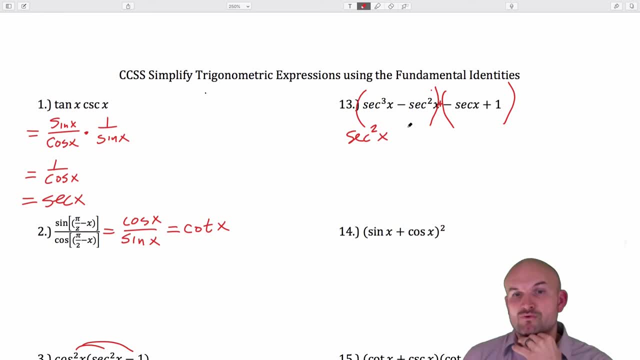 Now I'm going to factor out my common element here, which is secant squared of X. And when I factor out a secant squared of X, I'm going to be left with a secant of X minus one, And then here I can factor out a negative one. 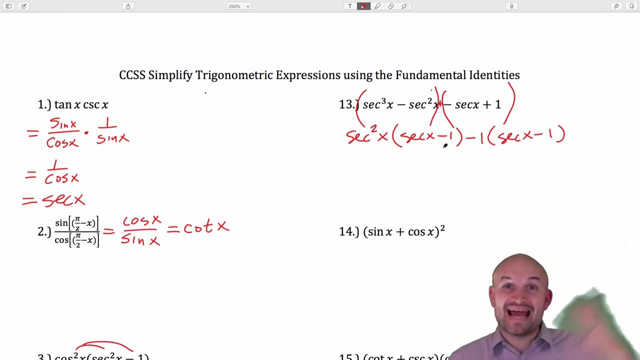 So, therefore, that's going to give me a secant of X minus one. Now I can factor out the secant of X minus one, And that's going to be leaving me with a secant squared of X minus one, which again is going to be equal to a tangent of X. 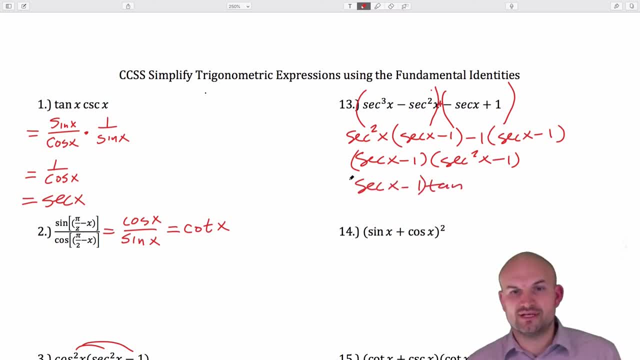 So you minus one times- oops, let's put that in parentheses- times a tangent squared of X. right, Because remember the Pythagorean identity. you know, tangent squared of X plus one equals secant squared. Now again, you could distribute that. 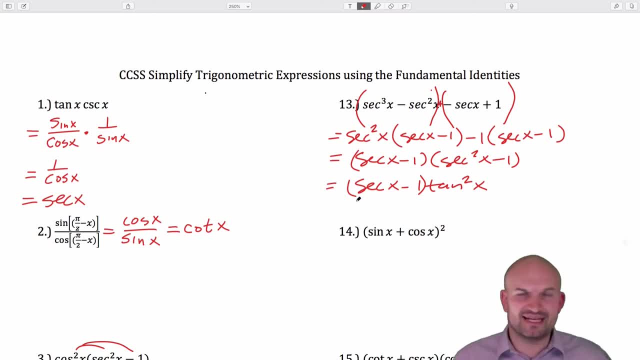 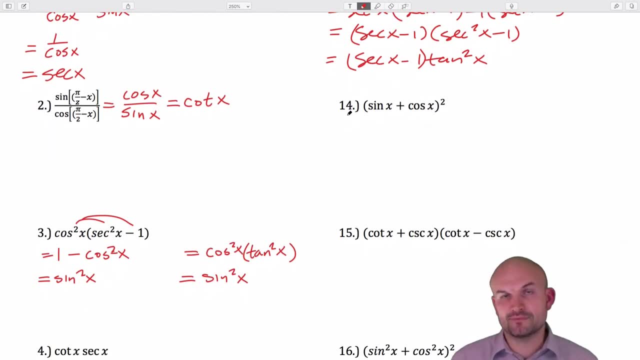 But you know I'm not really seeing how that's going to make anything you know easier or more simple. The next example: So typically you know kind of a good rule of thumb: If you know the operation has a multiplication like something being squared or multiplication like 15, you're going to want to apply the operation. 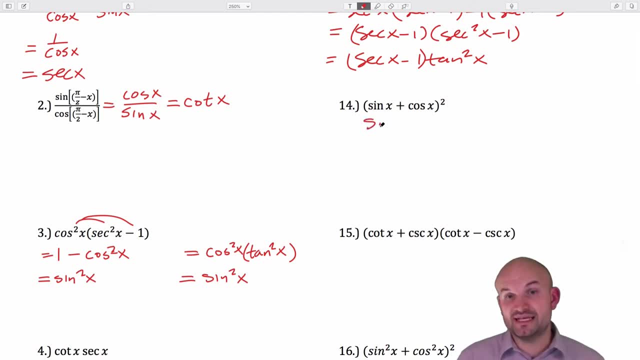 Now remember: sine of X times cosine of X just means that sine of X plus cosine of X times the sine of X plus cosine of X, right? So we need to go ahead and apply distributive property. That means basically multiplying everything times everything. 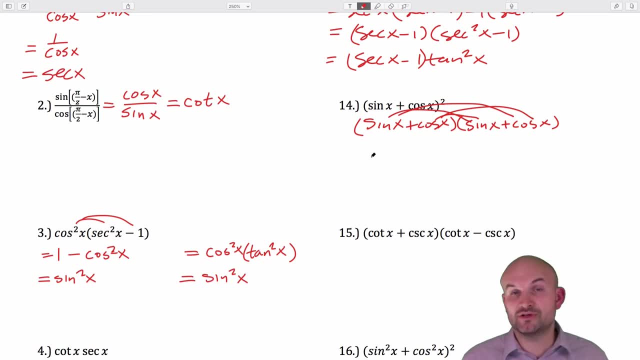 Hopefully you recognize, though, when you have a binomial squared, that's going to produce a perfect square trinomial. So I have a sine squared of X plus a two sine of X, cosine of X plus a cosine squared of X. Now hopefully you recognize that we have sine squared of X plus cosine squared of X. 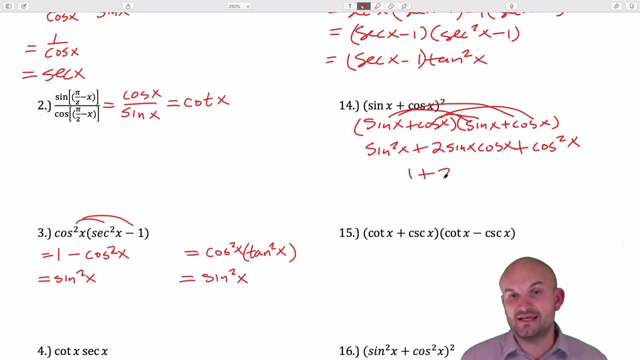 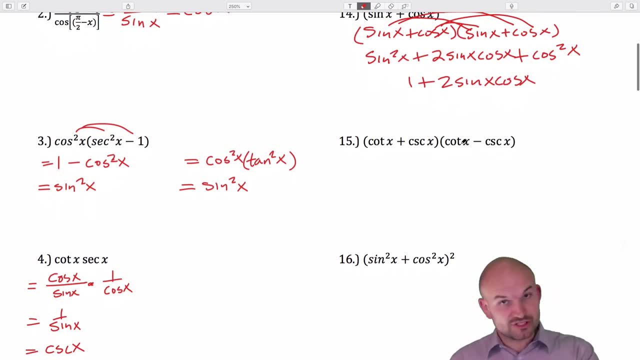 That's going to equal one right Being your Pythagorean identity, And then we'll have a two sine of X, cosine of X. okay, In the next one, you could go ahead and multiply using the difference of two squares. However, since these are the exact same binomials, except one's positive and one's negative, 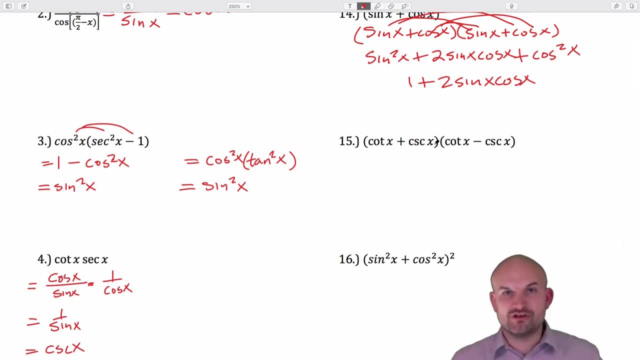 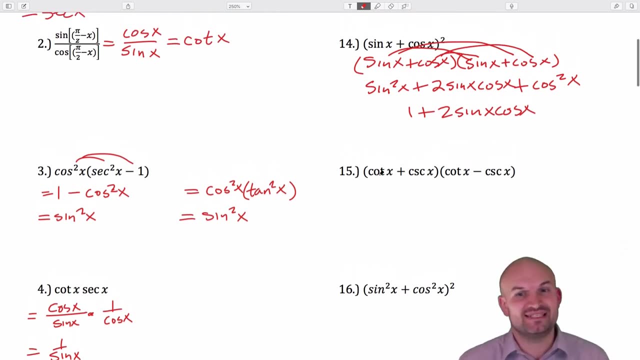 in this case, when I go ahead and distribute, I recognize I'm going to have a difference of two squares, Meaning instead of my middle terms combining to give me two, my middle terms are going to combine to give me zero. So I can just follow the formula for difference of two squares and just square the first two terms and square the second two terms. 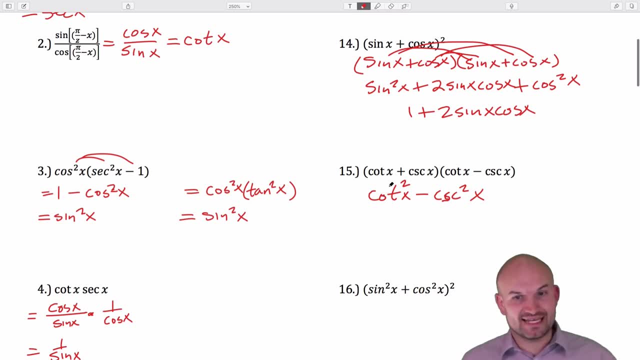 Now I can identify my Pythagorean identities again and say: oh yeah, You know, cotangent of X plus one equals cosecant. So therefore, if I subtract the one, I could say that cotangent is going to equal cosecant squared of X minus one, minus cosecant squared of X. 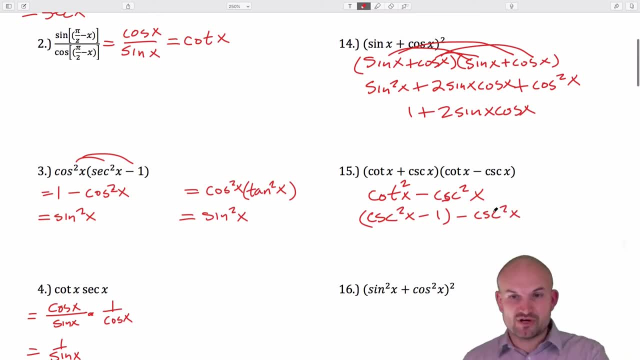 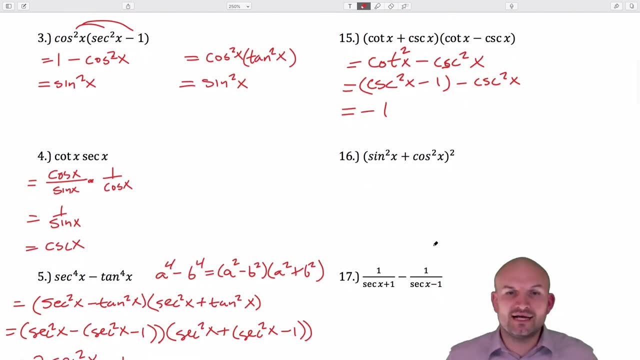 And now you can see that cosecant squared of X is going to subtract from cosecant squared of X, which is just going to leave us with the number negative one All right On to number 16. here, In this case, you see that you have sine squared of X. 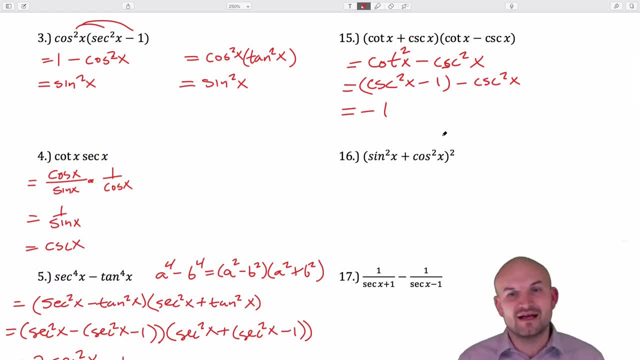 Sine squared of X plus cosine squared of X. Instead of multiplying, you just recognize: oh, that's equal to one. So you have one squared which is just equal to one Kind of nice right. All right, The next one gets into a fraction. 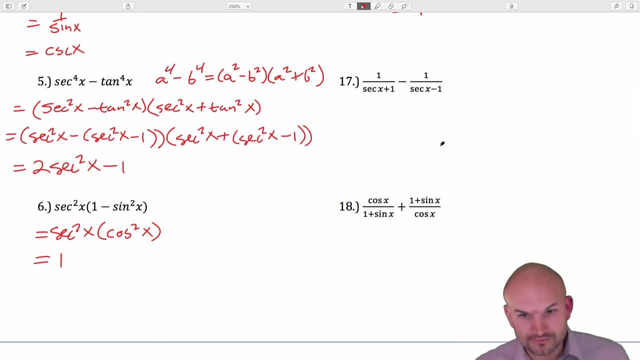 Is that the easiest fraction I gave myself? It is Geez. So remember when we're adding fractions here. basically, what we want to do is make sure that we have common denominators, And in this case, you can see that we do not have a common denominator. 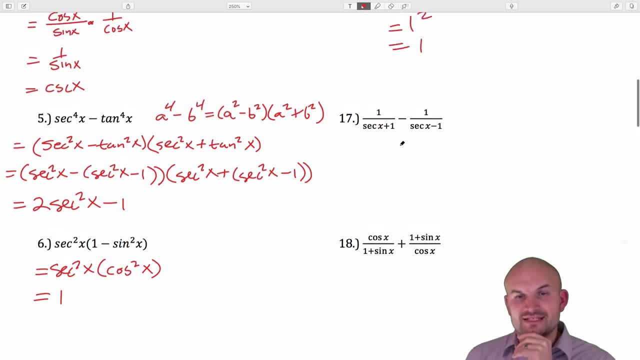 So what we're going to want to do- I'm sorry, up here- is say: all right, since these don't have any common. the easiest way to identify common denominators is just to multiply by the other denominator on the top and the bottom. 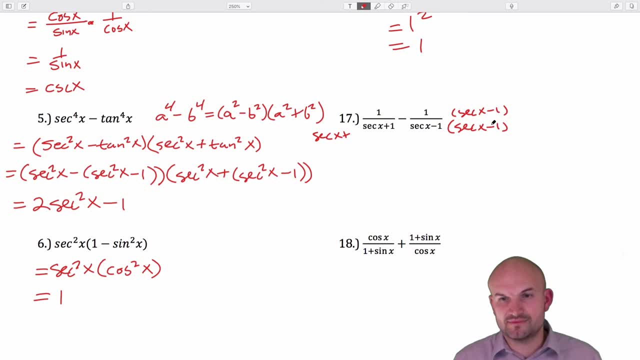 So we have secant of X, That's plus one- I'm sorry, Geez- And then this would be secant of X minus one And then times the secant of X minus one. Okay, So when you multiply on the top, on the left, here on the right, 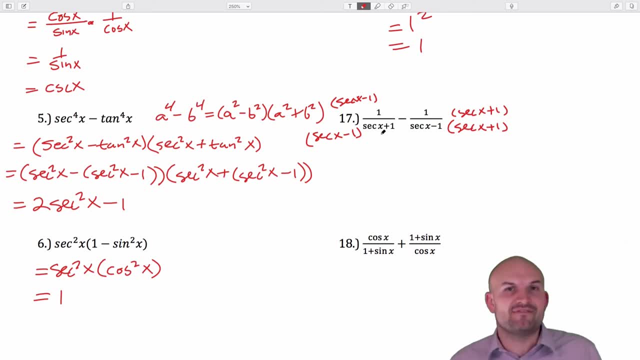 And, again, that's because these do not have any common elements. Yes, they have a secant of X, but it doesn't evenly divide into either of them. So when I combine these, though, I'm going to have my common denominator, which is going to be secant squared of X minus one. 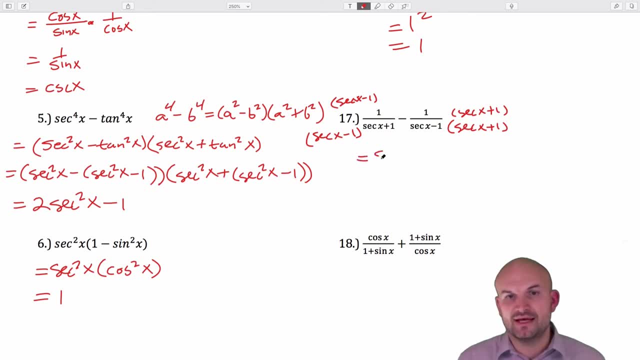 And then my numerator. I'm going to have a secant of X minus one, right times one, And then minus- make sure you use parentheses here- A secant of X plus one. Okay, So my common denominator is a secant squared of X minus one. 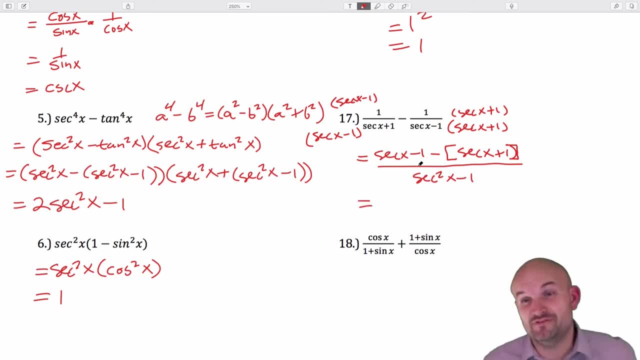 Now, hopefully you recognize that is a Pythagorean identity that's going to give you tangent squared, And then you recognize here that the secants are going to subtract out, And then I'll have a negative one minus one, which is a negative two over secant squared of X minus one. 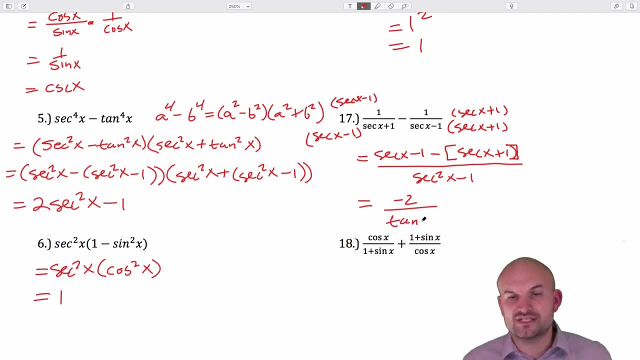 So secant squared of X, that's going to be a tangent squared of X, And now I could rewrite this. without question, I could rewrite this, without being the denominator, as a cotangent squared of X. All right, So for the next one, again, we kind of have the same idea. 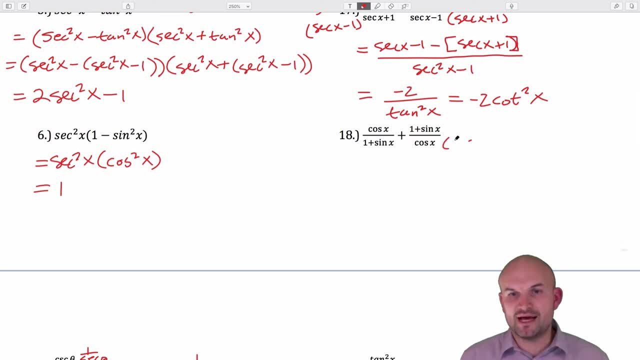 These denominators do not have anything in common, So therefore I'm just going to multiply by the other denominator to go ahead and simplify. Okay, So on this left-hand side I have cosine squared of X, And then that's going to be plus. 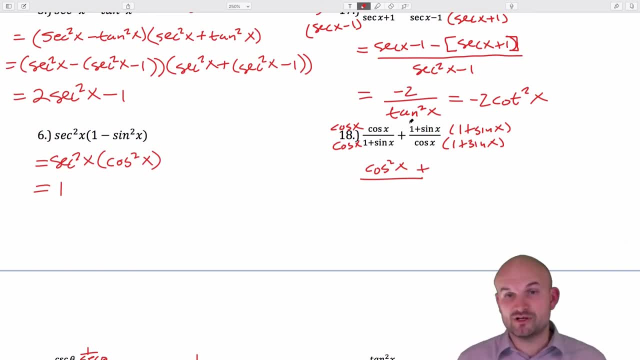 Now this I'm going to have to expand out. I'm going to have to recognize, though, again, this is a perfect square trinomial. So therefore it's going to be one plus two, sine of X, plus sine squared. 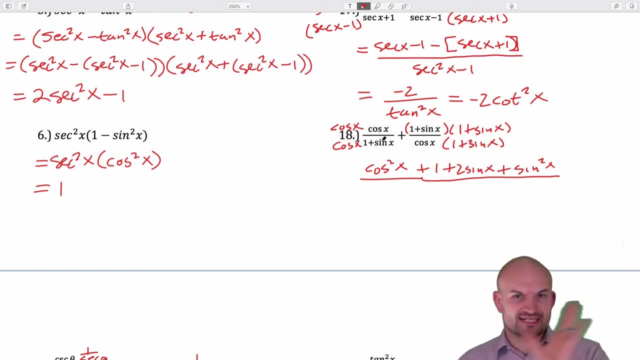 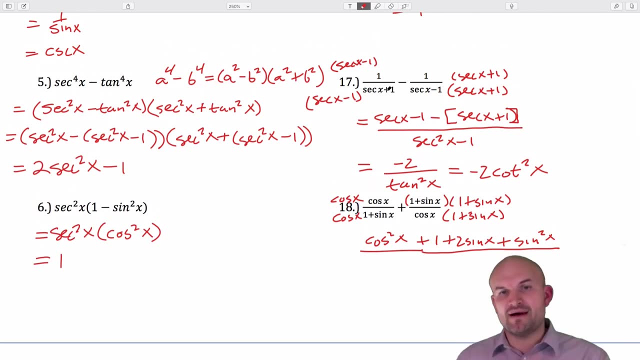 All right, Now, in this case I'm not going to multiply the cosine times of one plus sine squared. So in this case I multiplied these denominators because I knew they were going to provide me. Whenever you have a binomial multiplied by its conjugate, it's going to produce your Pythagorean identities. 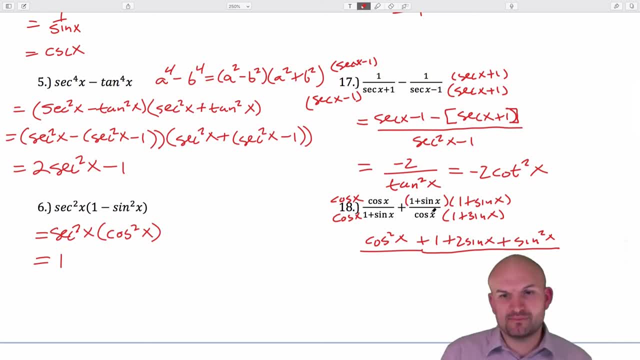 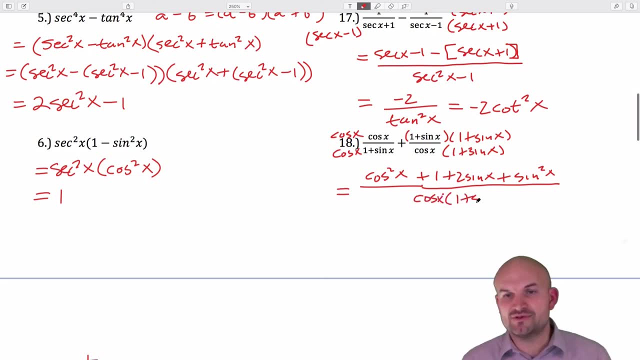 In this case, this is not going to produce a Pythagorean identity, So I'm going to leave this just non-multiplied out, because I don't see how multiplying it through is going to actually simplify my answer at all. However, I recognize cosine squared of X plus sine squared of X is going to equal one. 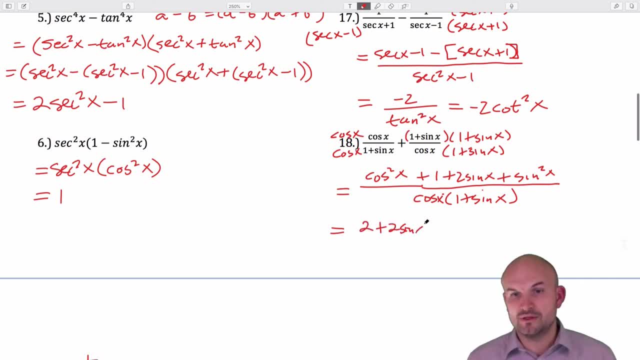 So then I have: one plus one is two plus two, sine of X, all over a cosine of X times one plus sine of X. Now hopefully you see that in the denominator I can factor out a two, And that's going to leave me with a one plus a sine of X all over this cosine of X times one plus the sine of X. 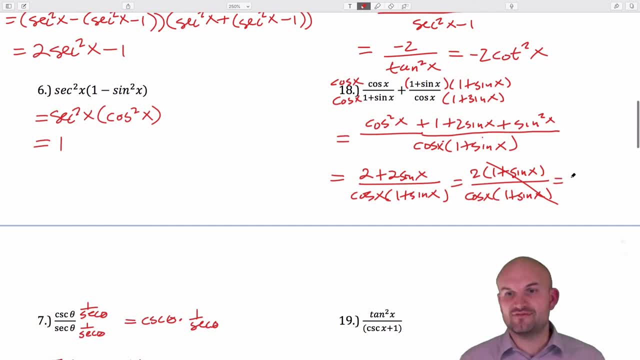 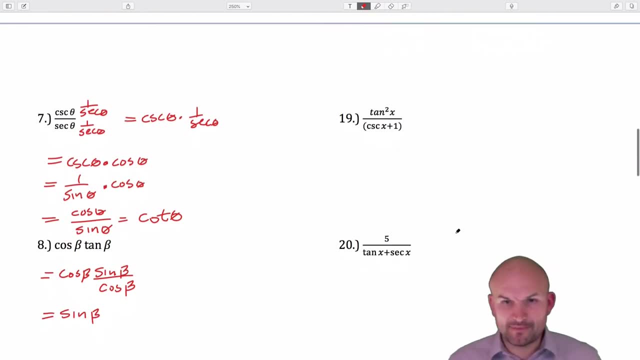 Now everything's separated by multiplication, So those are going to divide out And that's going to leave me with a two secant of X. All right, So for the next example. now again, here kind of comes into this interesting point here. 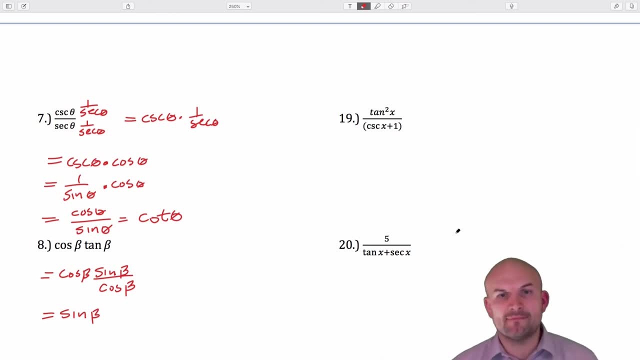 I have the cosecant of X plus one, And what I'm trying to obtain here is I want to like somewhat simplify this Right And I can't like simple straight divide that into it, you know, into tangent squared. So one of the key, one of the key important items that we want to look into is is creating these Pythagorean identities. 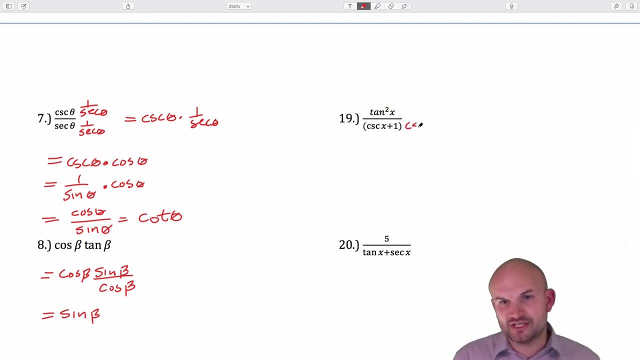 So if I multiply by the conjugate cosecant of X minus one, If I multiply by this conjugate, what that's going to do is that's going to create a Pythagorean identity here in the denominator. So therefore I have a tangent squared of X times a cosecant of X minus one, all over a cosecant of X minus one cosecant squared. 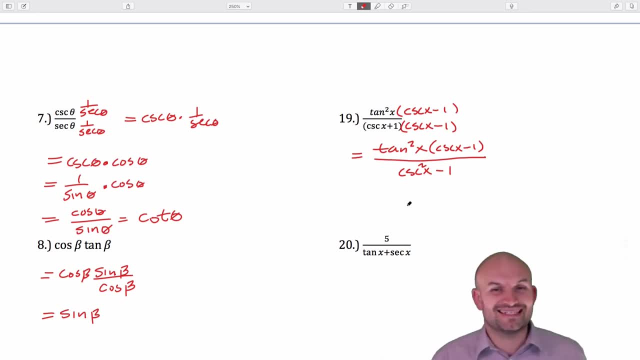 Sorry, of X minus one. Now, looking at my Pythagorean identities, that's going to leave me with a cotangent, So I'll have a tangent squared of X times a cosecant of X minus one, All over a cotangent squared of X. 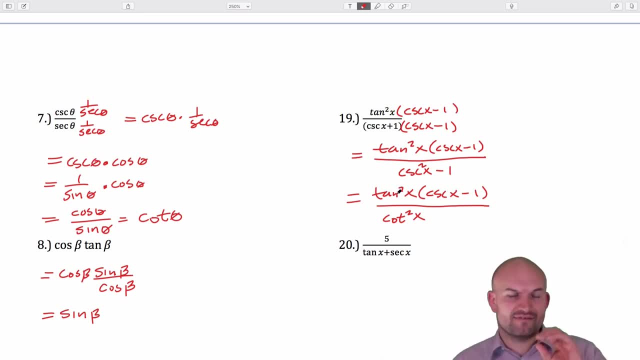 Now remember This is like having tangent divided by cotangent or so. Therefore, if I was going to multiply by my reciprocal here, I'd multiply by tangent squared on the top and the bottom. So that's going to leave me with a tangent to the fourth times, a cosecant of X minus one. 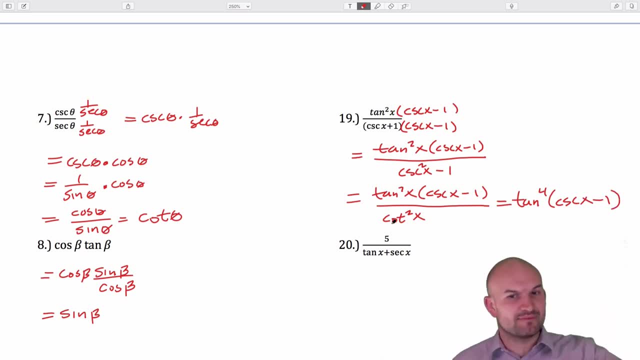 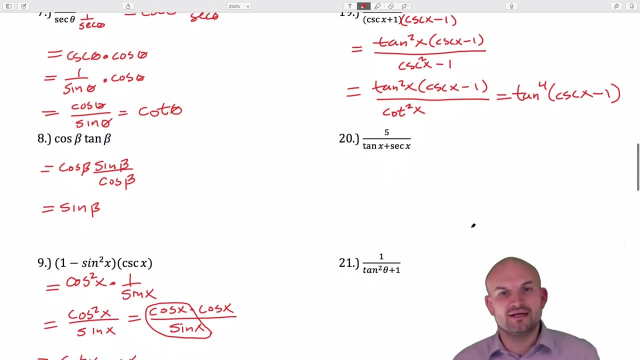 Okay. So again, basically, what I'm doing is, instead of dividing by cotangent, you can multiply by the reciprocal, which I kind of ran on. I'm going to give you a little bit of space here, But you can see, that would give you tangent to the fourth. 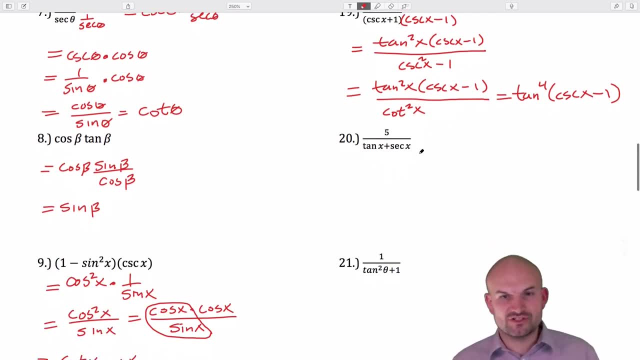 Now for the next example, number 20,. that's the same thing we have here, Like there's nothing else I can really do to divide tangent of X plus secant of X into you know five. So what I'm going to do is I'm going to multiply by the conjugate. 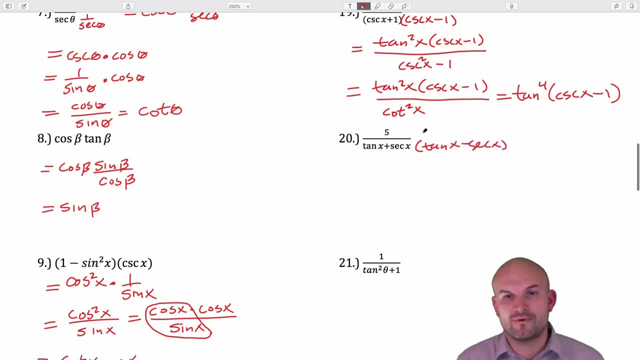 So let's go ahead and create that. So we have tangent of X minus secant of X, And we're just going to do this on the top and the bottom. Now I could multiply it, distribute the five, But I'm just going to leave that out for a second. 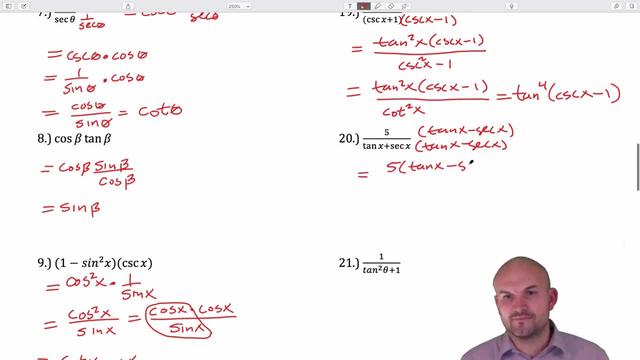 Let's just see what's going to happen here. All right, So in the denominator here I'm now going to have a tangent squared of X minus a secant squared of X- right, Because this is a difference of two squares. And then I could rewrite secant squared as tangent of X minus one. 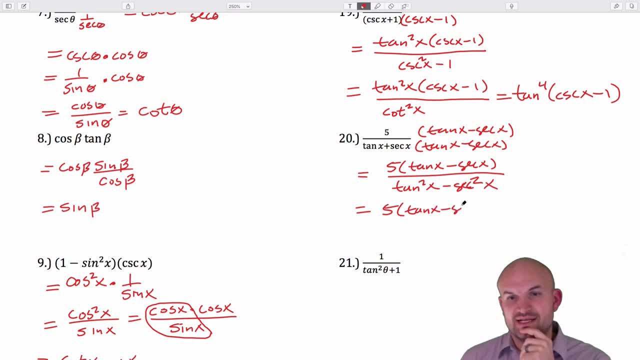 So I have five times tangent of X minus secant of X All over tangent squared of X minus tangent squared of X minus one. I'm sorry, Secant, yeah, Secant is going to be tangent squared of X minus one. Well, what you notice here is this becomes a positive one. 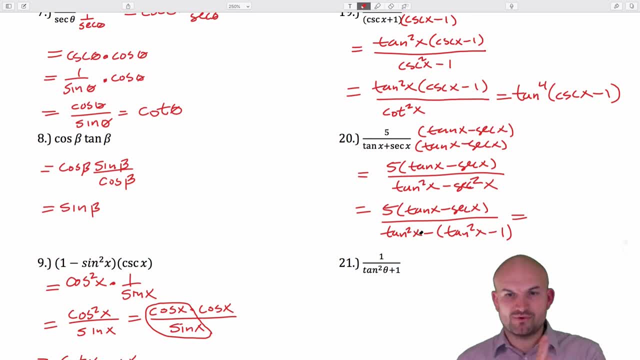 This is just going to. that's going to go to. so tangent squared of X minus tangent squared of X goes to one, And then we're subtracting a negative one, which is going to be a positive one. So that gets rid of my fraction. 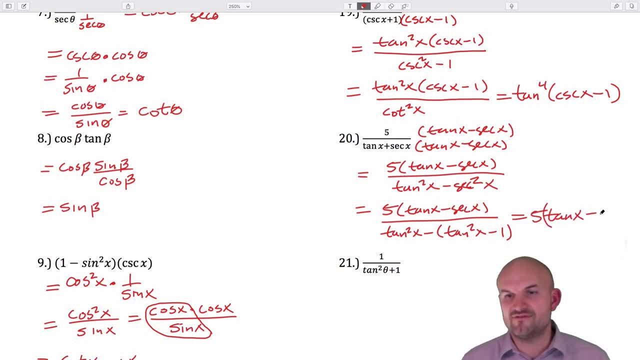 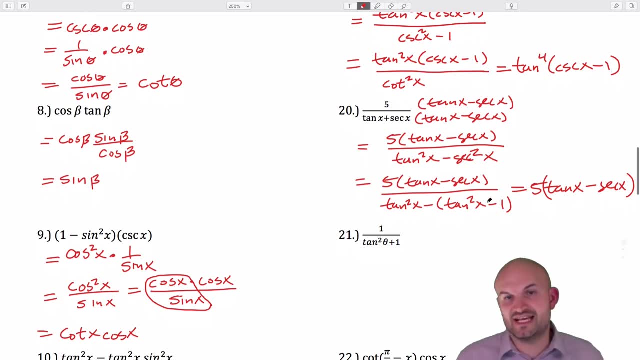 So I have a tangent of X- Let's put the parentheses there- Five times a secant, Five times a secant of X. So you can see, at least that got rid of my division of tangent of X plus secant of X. 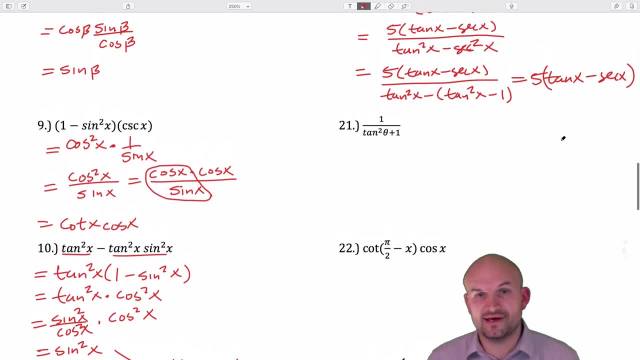 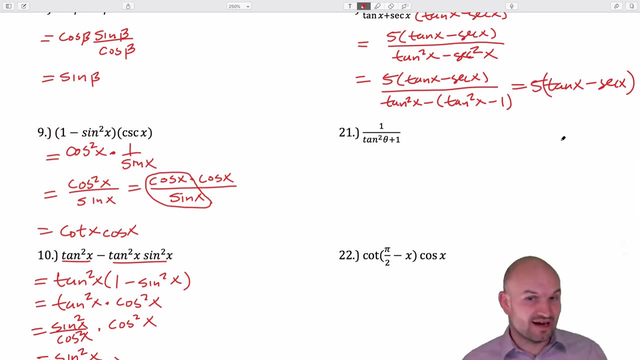 Did I do that? Yeah, I need another example of that, but that's kind of a difficult problem, All right. So in the next example I have one divided by tangent squared of X, tangent squared plus one. Hopefully you recognize that tangent squared of theta plus one is equal to secant of theta. 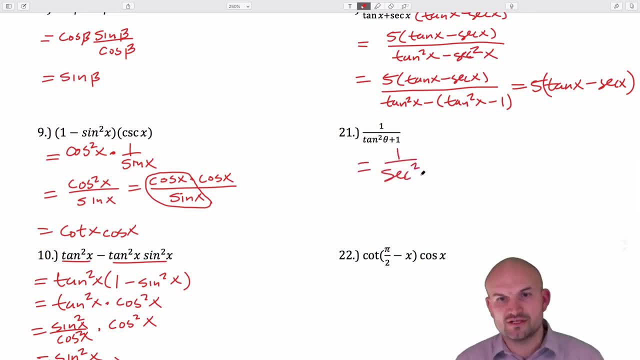 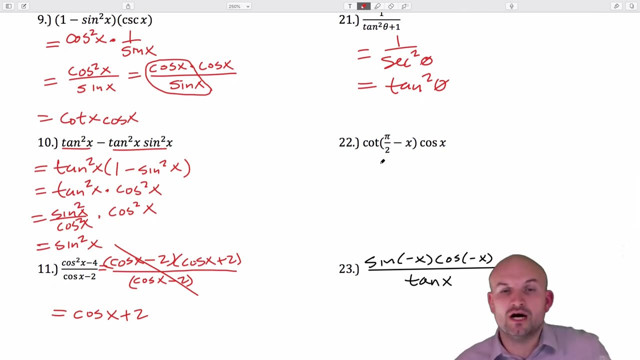 Well. so therefore, I can rewrite this as one over secant squared of theta. Well, again, one over secant squared of theta. using your reciprocal identity is just going to equal tangent squared of theta. The next one is again another opportunity for our co-function identity. 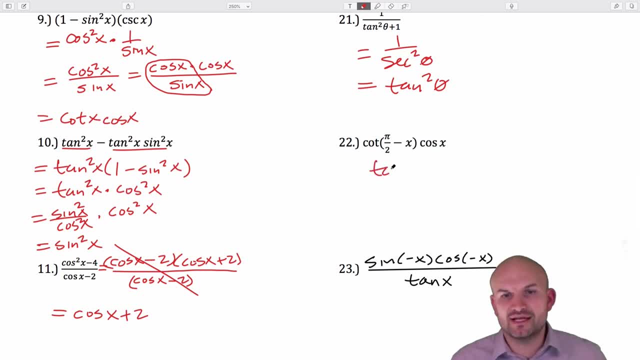 So I see the cotangent of pi half minus X times cosine. So again, using my co-function identity, that's going to be tangent of X times the cosine of X. And remember, tangent is sine over cosine, So therefore this can equal the sine of X. 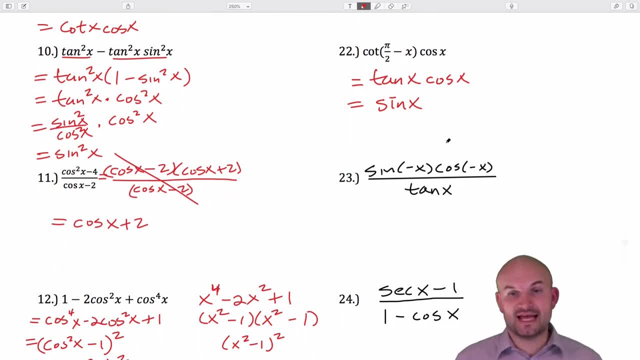 The next one. I'm going to use my even-odd identities And remember that when you have the even-odd identity for sine of negative X, that's going to equal a negative sine of X times a cosine. But however, the cosine of a negative angle is actually just equal to cosine of X. 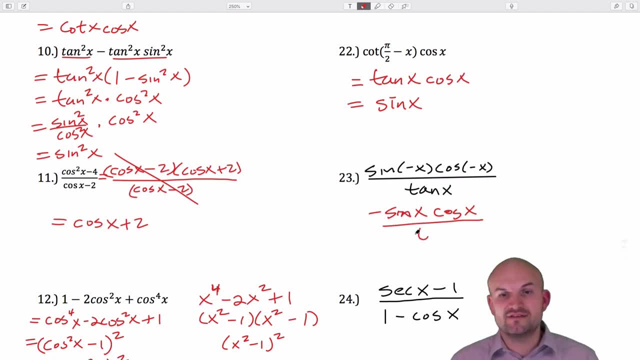 Again, these are from your even-odd identities, divided by the tangent of X. Now again, instead of multiplying by the tangent of X or dividing by a tangent of X, I'm sorry, we could go ahead and multiply by cotangent or cosine. over sine right. 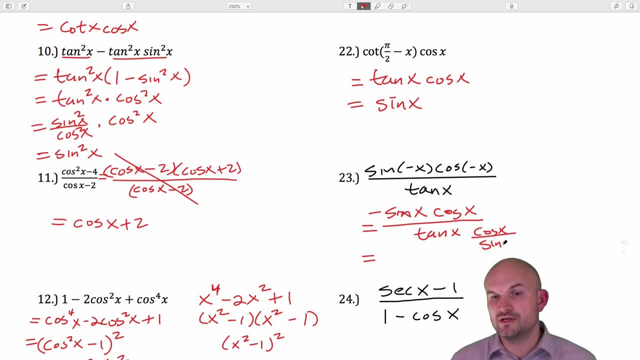 So what I'm going to do is I'm going to multiply by cosine over sine of X And hopefully you see here that the sines are going to divide out and the cosines will square. We'll multiply by each other. So therefore it's going to be a negative cosine squared of X. 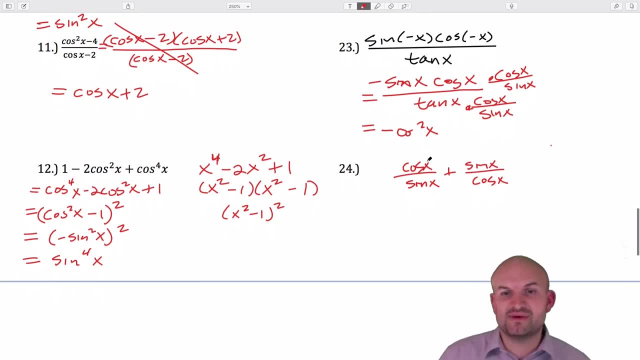 Okay, so onto our last problem here. In this case, we have cosine of X over sine of X, plus sine of X over sine of X, And I probably should have done this one before the other ones that we were trying to add our fractions to. 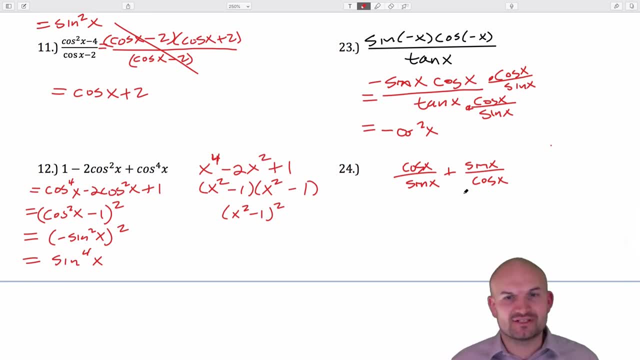 But again, here you can see that again. another example where we have two fractions that do not have anything in common as far as their denominators. So to go and combine them, I need to have a common denominator. So again, since they don't have anything in common, I am just going to multiply by the other denominator.